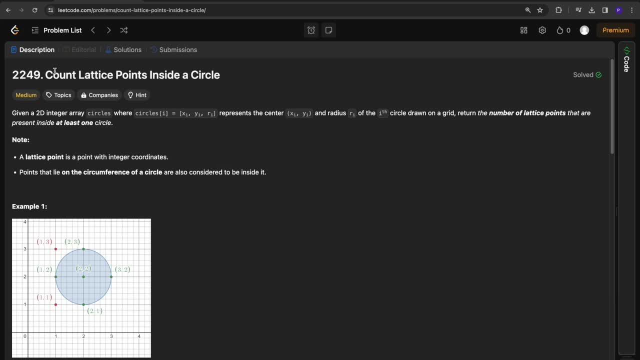 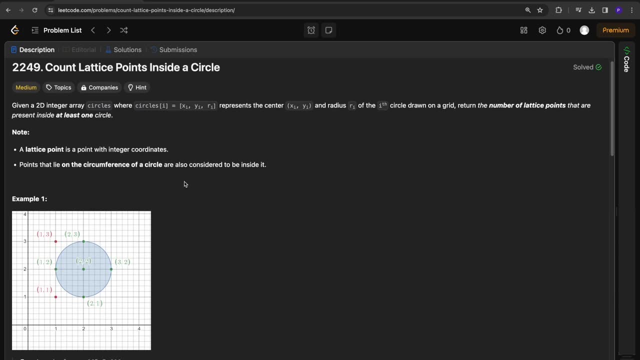 In today's video we are going to solve count lattice points inside a circle problem. So in this problem they will give a list of circles and we need to find how many lattice points are present. So a lattice point is a point which has coordinates as integers. So if you consider this, 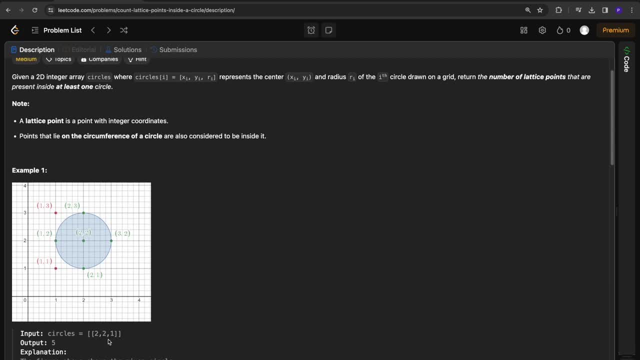 first example: they have mentioned only one circle. So they have mentioned first two numbers which are present in that vector represents x and y coordinate of the center, and the next number represents the radius of that particular circle. So if you consider this circle in this image, so 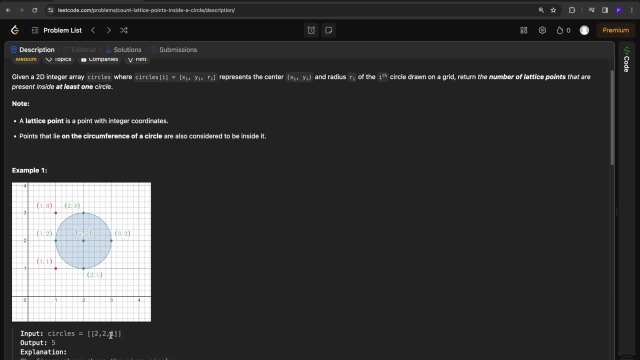 2 comma, 2 is center, So that is what is given here, and 1 is the radius of the circle. So we need to find out how many lattice points does belong to this particular circle. So from the radius, if you consider these points, 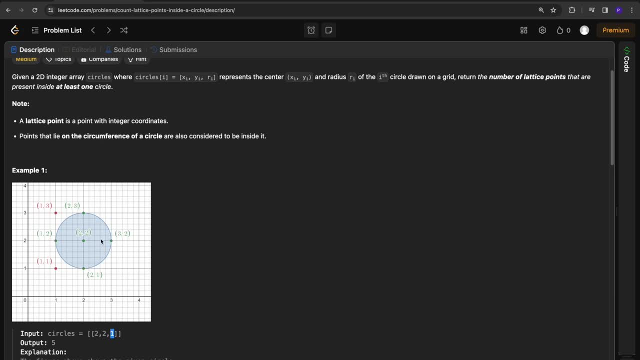 1, 2, 2, 3, 2, 1 and 3, 2 only including this point totally, there are 5 points: 1, 2, 3, 4 and 5.. So there are 5 lattice points which are present inside this circle. So inside, in the sense, even if the 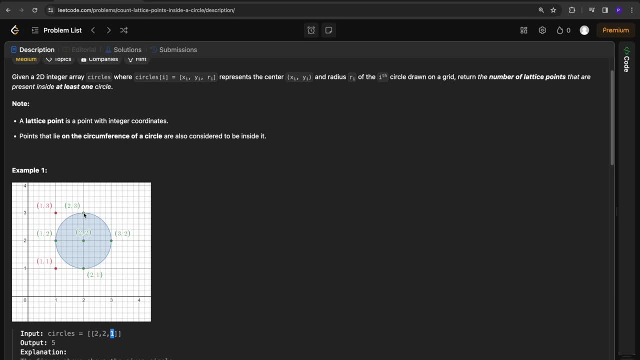 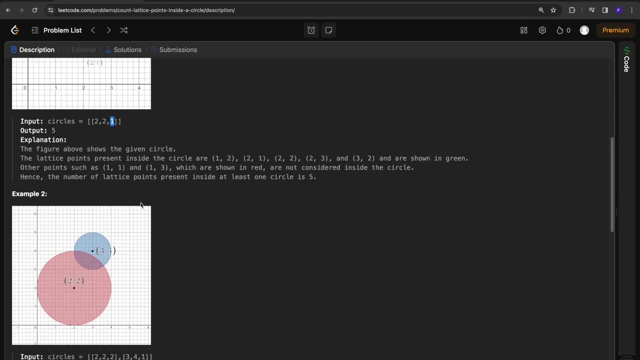 point is on the perimeter of that circle, that will be included. So we need to find out all such points and we need to return the count of such points. So if there are more than one circle, then at that point we need to find out how many lattice points are present inside that circle. So 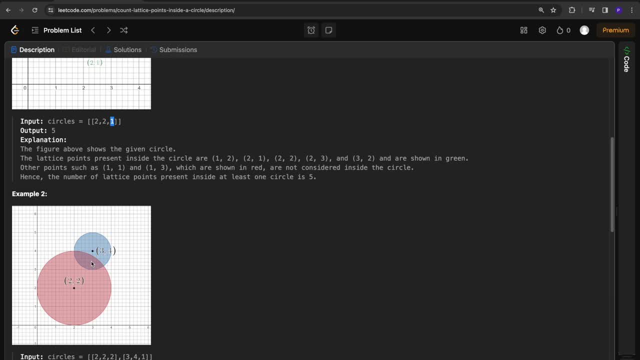 to find out those 16 lattice points. we don't have to double count a particular point. Let's say, if let's consider this point, if the point which is present at the intersection of circle 1 and 2. And if a point belongs to both the circles or multiple circles, it has to be counted only once. 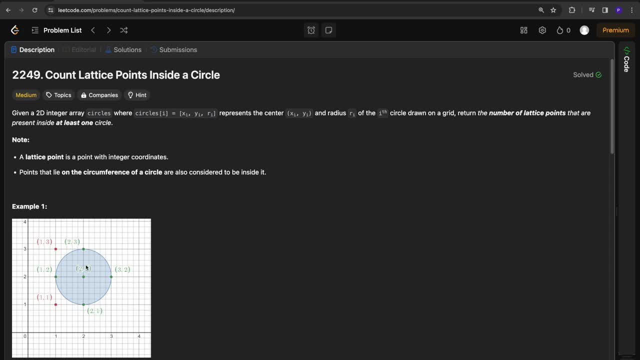 So intuition is very simple here. So what we can do is let's say: if this is the center, center coordinates are x and y, And at max x coordinate can go from x to. if x is a center, then leftmost coordinate will be x minus r. 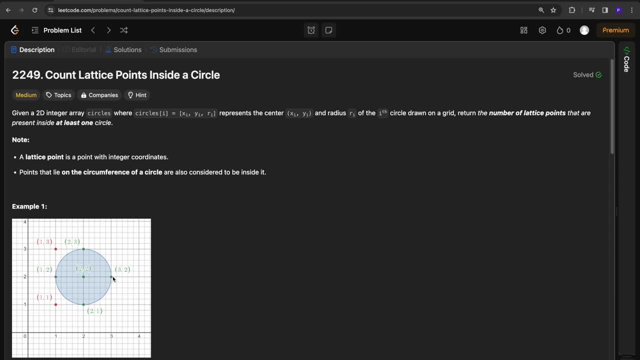 because this is a circle and the rightmost coordinate will be x plus r. R is the radius of the circle and the topmost. if y is the y coordinate of the center, then topmost coordinate of that particular circle will be y plus r and similarly like bottommost. 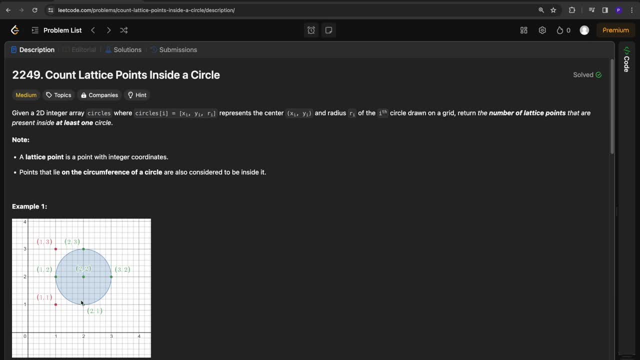 lattice point for that particular circle will be y minus r. So if we keep this intuition and if we can iterate over all such points, and if we can decide if that particular point belongs to the circle or not, then we can keep easily keep count of those points. Let us implement the same. 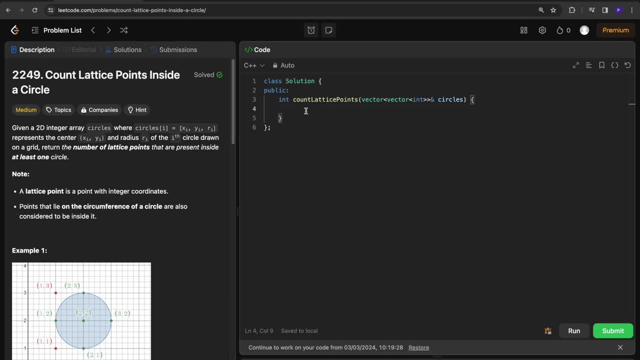 solution so that this explanation becomes available. So let us start with going through all circles. for int i equals to 0 and i less than circles, dot size i plus plus. So now we are at a particular circle, we can extract x, y, and so let us say center. 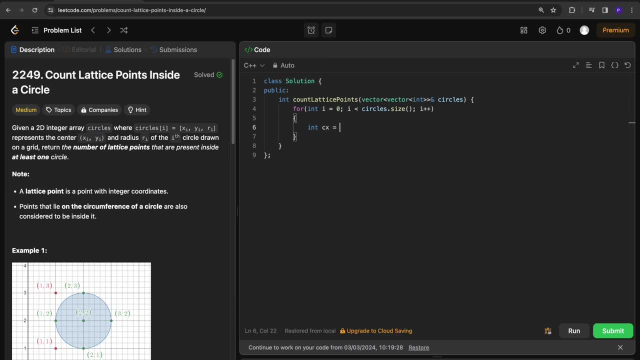 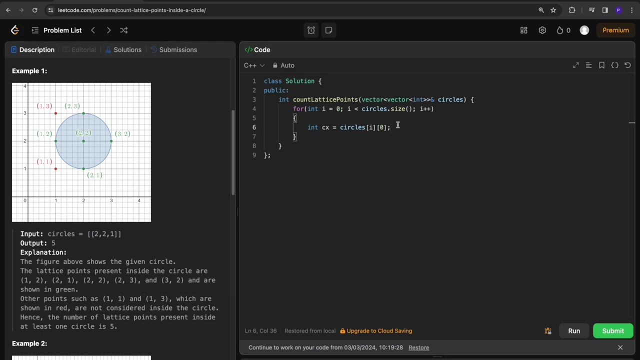 circle, center x. So cx represents the x coordinate of the center. So cx will be equal to circles of i, that is the circle that we are considering- and at 0 the first element will be x, coordinate of the center, and similarly int cy, which represents the y coordinate of the center of the circle. So 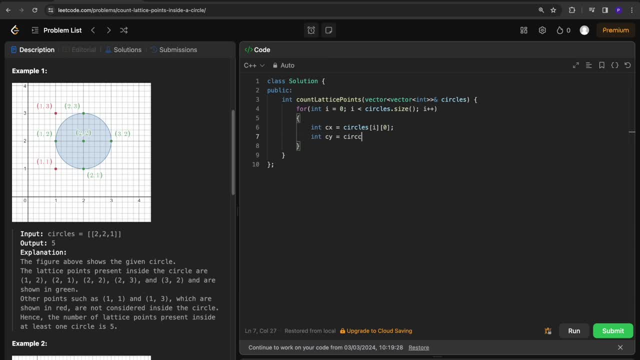 that will be circles of i of 1.. So now we have x and y coordinate of the center, and another thing is the radius, that will be circles of i comma 2.. So now we have extracted these parameters that are given to us in this circles argument. 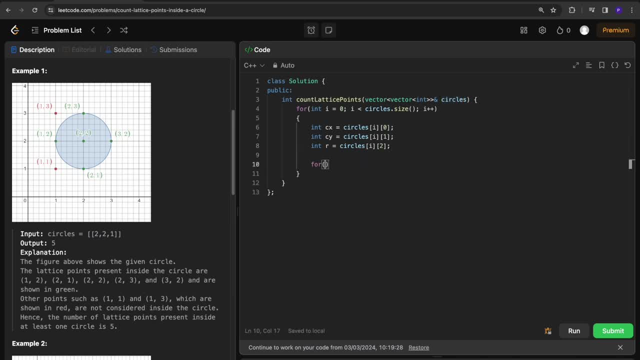 And now we just have to iterate over the range For int. x equals to x, range will be cx minus x, So that is the leftmost range. Let us say: if this is cx, this will be c minus cx minus r, actually cx minus r. that is the radius, r is the radius. So from x will range from here to, and x is less. 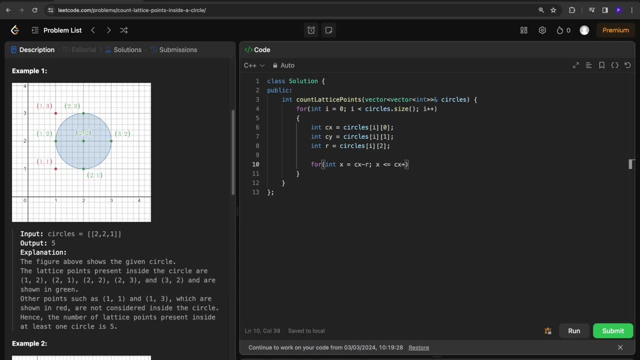 than or equal to center x plus r. We can iterate over this range And similarly for y, y will range from: if c? y is the y coordinate of the center, then the bottom most is c? y minus r. So c? y minus r and y. 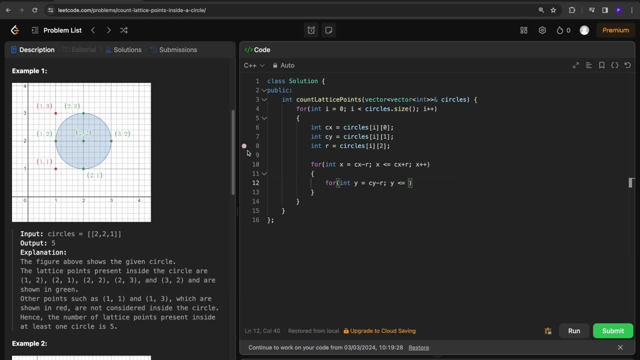 less than or equal to the topmost value will be cy plus r. this plus and minus r comes from the properties of the circle and we can iterate over these points and then we have to check if this particular point, that is the point, current point that we are considering, x comma y. 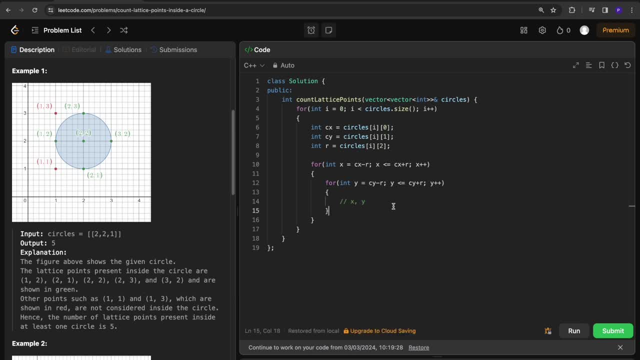 whether this belongs to our circle or not. so that can. for that we can make use of the distance formula. so if you want to find out difference between distance from the center, we can make use of the distance formula. and from that distance formula, let's say if 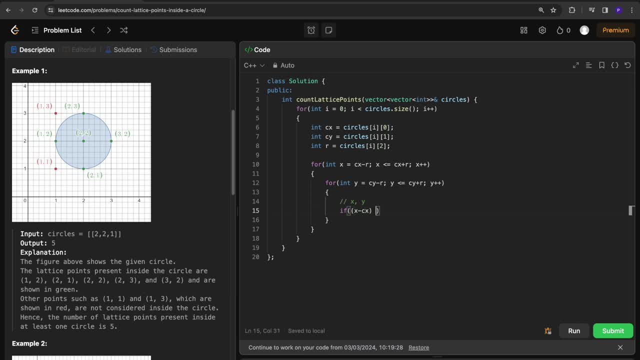 if x minus cx multiplied by x minus cx, you c x plus, then y minus c y multiplied by y minus c y. So if this particular distance is less than or equal to radius square, so that is r multiplied by r. if this is the case,